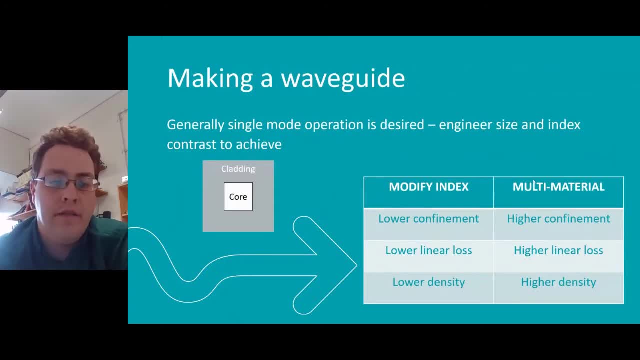 different regions in one of two ways. The first way is to make both core and cladding distributions out of the one material and then perform some operation to modify the refractive index, And the second option is that we can use multiple materials for this. 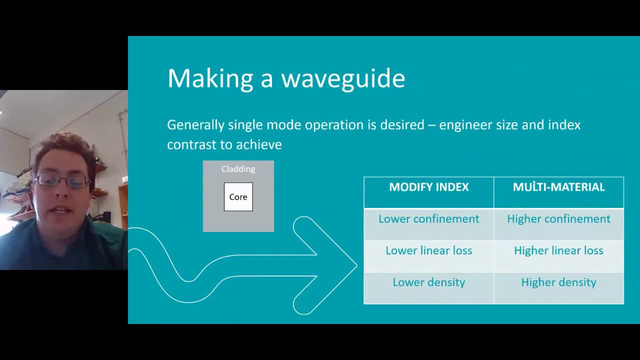 structure. Generally, if we're using multiple materials, the refractive index contrast will be higher, And that means that the waveguide will have a higher confinement, which can lead us to a higher integrated integration density, But usually also a higher loss per unit length, compared to those waveguides made by changing. 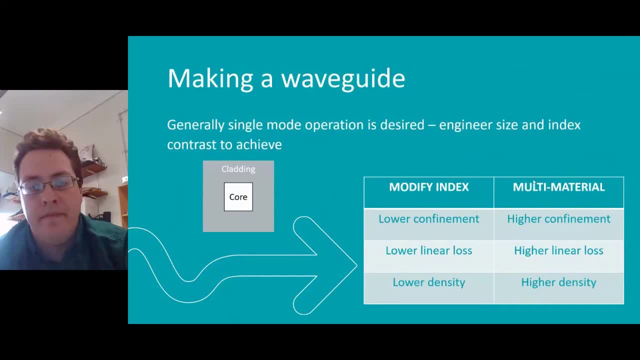 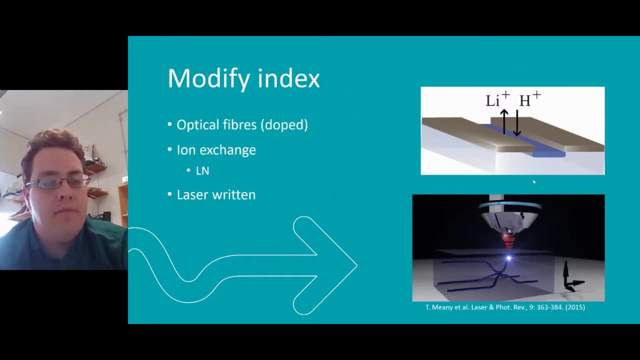 the refractive index of a region of a single material. So waveguides that are made in this method. there's a whole variety, but I'll just highlight a few. So you can dope the material to change the refractive index, You can perform a line exchange process or some. 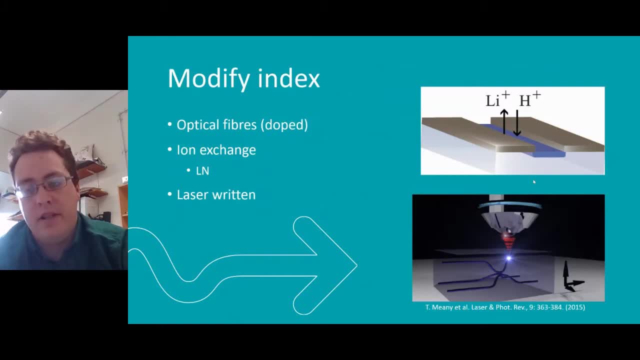 sort of chemical reaction to physically change the contents of the crystal structure. And the third option, quite often used in a lot of glasses, is laser written waveguides, where high intensity laser is focused into a small region, altering the structure of the material and changing its refractive index. 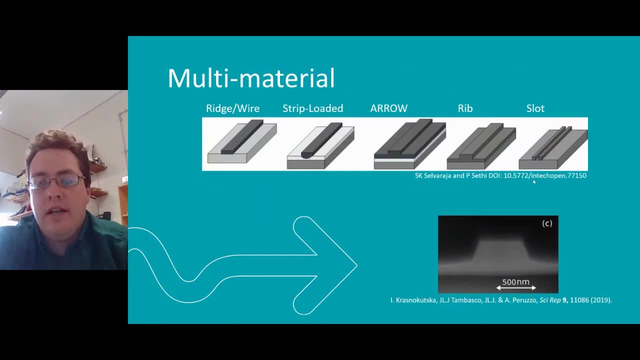 If we want to use more than one material, we can change the refractive index by changing the refractive index. So if we're using multiple materials, there's a whole variety of structures that we could think of to use to make this confined region, And I'll just in comparison. 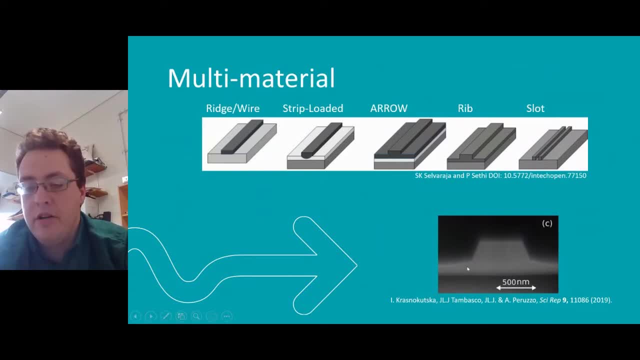 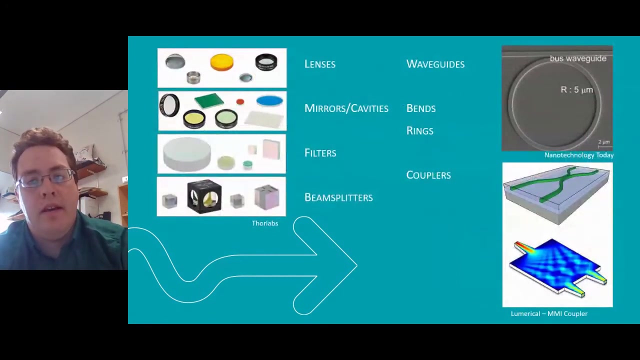 show, for instance, this image from the group of Alberto Caruzzo, where on the bottom we have silicon dioxide and on the top we have silicon dioxide And in between we have this sort of pizza hut roof shaped bit of lithium oxide. So, taking these waveguide structures, we want to look how we can implement everything. 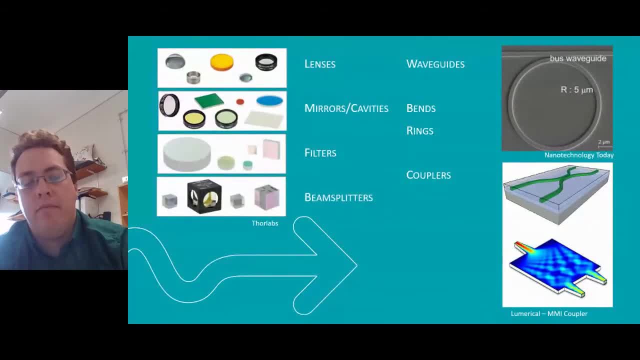 we can do in bulk optics in a integrated platform. So on the left I've listed the top four categories from Thorlabs where we've got lenses, mirrors, filters and beam splitters. When we're using waveguides, we can replace the lenses with filters and beam splitters When we're using 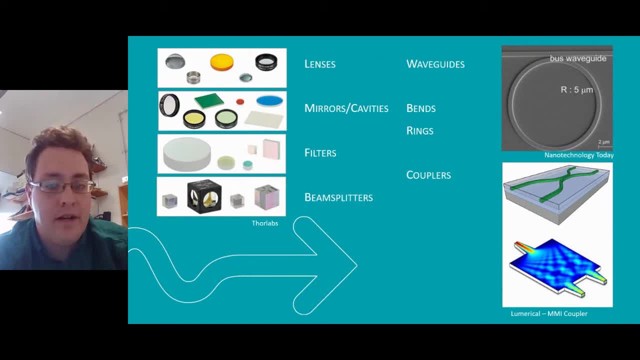 waveguides, we can replace the lenses with filters and beam splitters. When we're using ideal bucking même, we can use it as a perfect meet for mirrors, switches or even for polymers with straight waveguides and bends. If we want to make a cavity, we can continue bending. 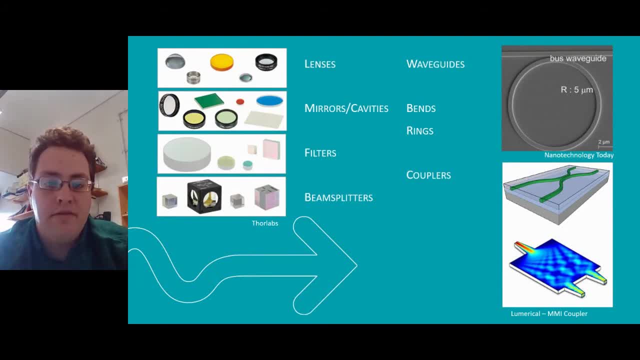 our waveguide round until we make a ring resonator. These ring resonators can also act as filters, but we can also use couplers as a type of filter as well, And these coupling regions can also be used for polarizing and non-polarizing. 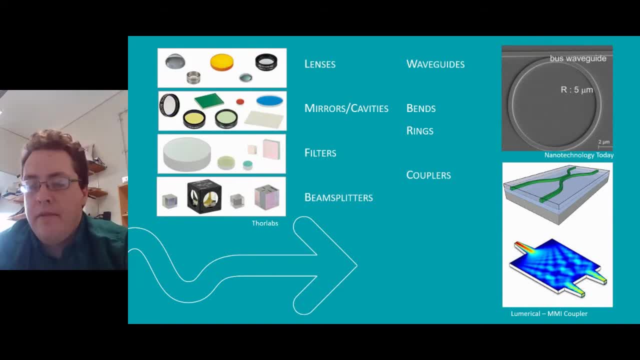 beam splitters, So a coupler. There's a poplar That's pure black. since it's high calibrated, No post pass. This coupler only лучes in the two main types, so normally you can have a. on the top there's a directional coupler. 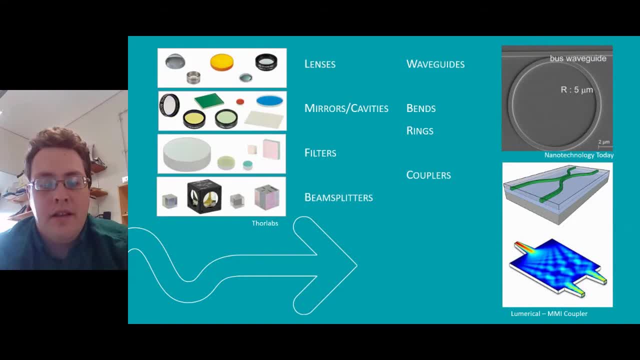 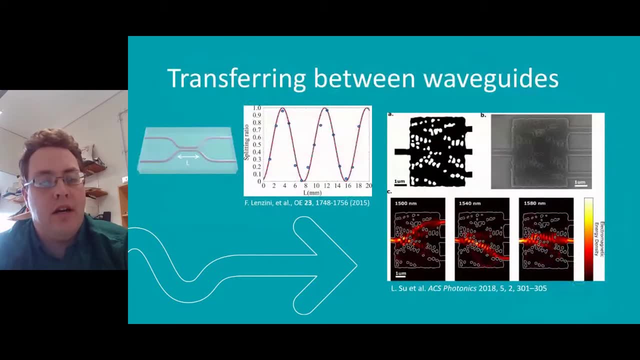 and on the bottom is a multi-mode interference coupler. so these are carefully engineered regions where we take a single or few mode waveguide and bring it into a region that's multi-mode and we engineer the interaction between these modes so that the output waveguides. 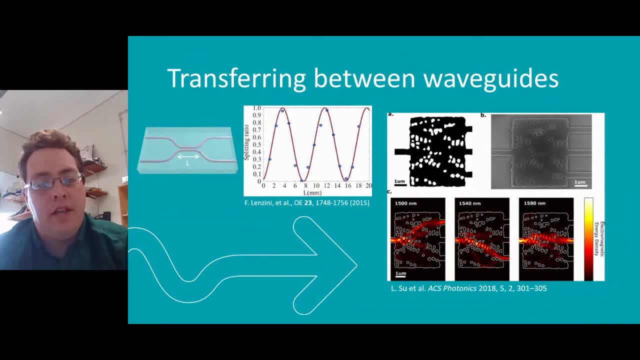 have some distribution of the input power. so in the case of directional coupler, we bring two single mode waveguides close together until they're evanescently coupled, and the length over which they're coupled and the distance between them changes how much light goes to each output. 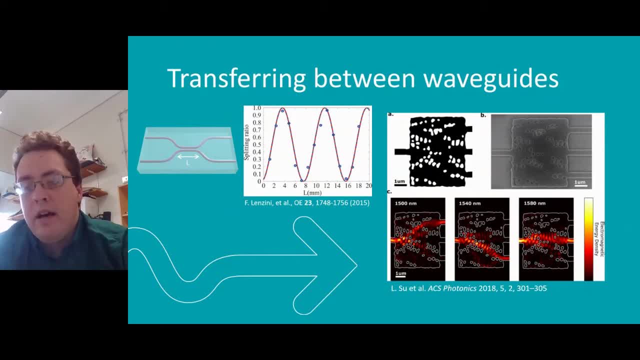 for a multi-mode interference coupler like the one on the right. we instead bring the light in through the input wave guide into a large slab of material where there's multi-mode interference coupler. we have a reference that's closer to the input And in mode propagation, and we can engineer the size of this slab so that we get the desired output. 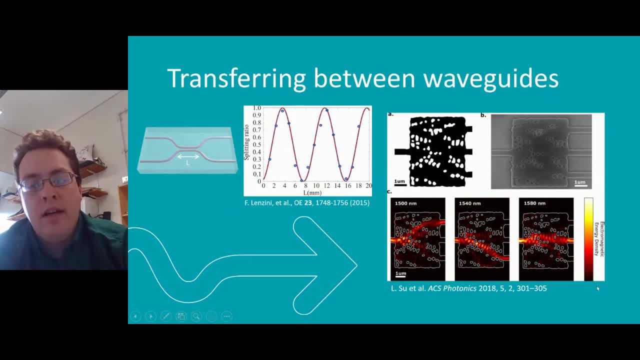 and we can do interesting things, like in this paper, where they've done some inverse design. so they've told the program that they want these three wavelengths of light to go to three separate outputs and then the program has given it, given them, a design to fabricate which to 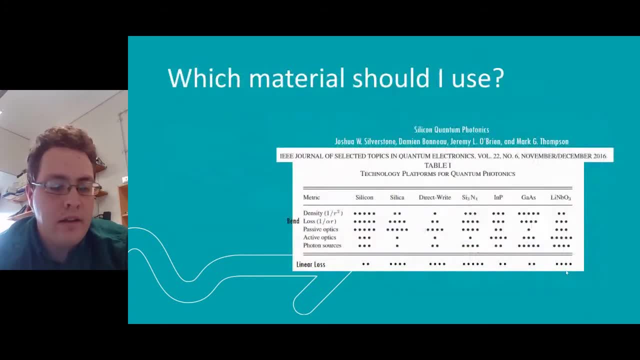 etch this particular structure. so the best way to decide which material you should use is really dependent on your application. i'll focus on just two here. the first is silicon. the usefulness of silicon is obvious, and the massive fabrication knowledge that we have for it gives us a huge advantage in terms of creating devices. 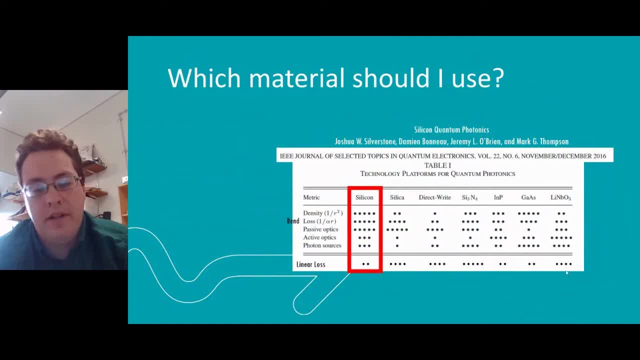 of a high complexity but unfortunately for some of these things we don't really have the desired properties that we want and it's difficult to engineer the right kind of reconfigurability and it's tricky to make them strongly non-linear. there's a lot of work going. 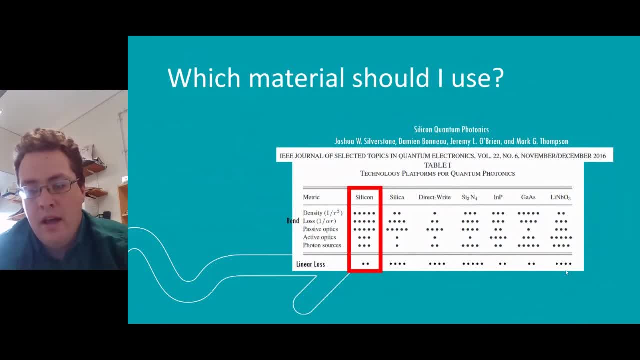 into this sort of stuff and they're getting great results um, but uh, sort of on the opposite side of the coin we have lithium nitrate, where we've got these great material properties, but we don't really have that um consolidated um fabrication expertise. so the materials that we're using um can be split up into two broad groups. one's called 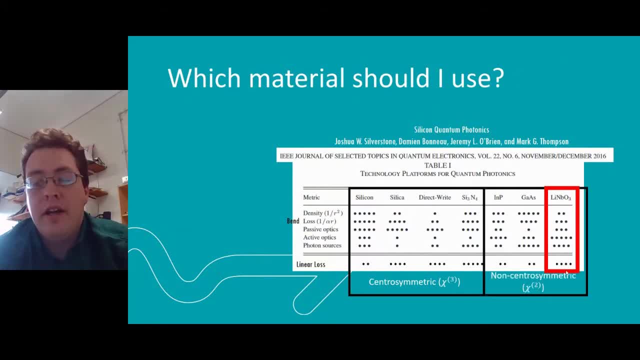 centrosymmetric and the other one's non-centrosymmetric, so centrosymmetry. all that means is that in the crystal structure, if you draw a plane of inversion through the center of the unit cell of the crystal, you get an inversion symmetry. so um, the symmetry of the crystal is. 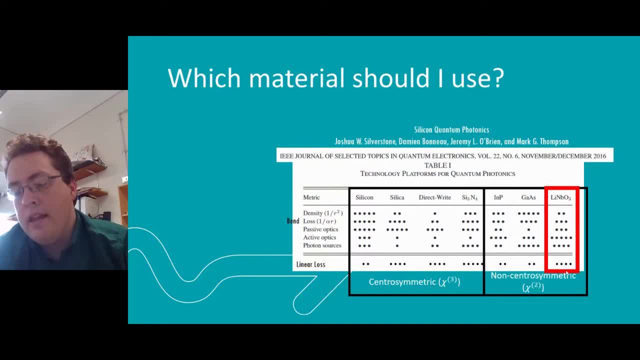 made a hundred percent split up into hieroglyph pieces. the symmetry of the silicon and silicon nitride fall into this category, and the non-centrosymmetric materials such as lithium nibe fall into this other category. and why this property of the crystal is important is because it determines 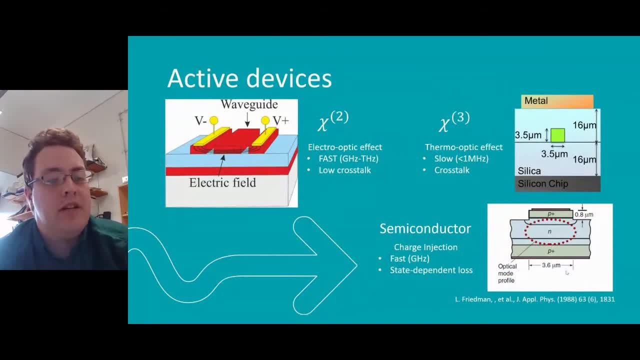 device in a Ki2 material, a non-centrosymmetric material like lithium niobate, we can use the electro-optic effect, where we apply an electric field to the waveguide and this changes the refractive index, and using this we can create phase shifters by simply changing the refractive. 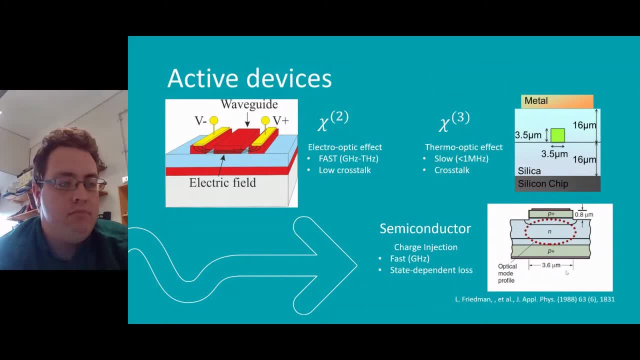 index of a certain length, or we can use it in these multi-mode coupler regions to modify how the coupler operates. In the Ki3, centrosymmetric materials like silicon, we can use instead the thermo-optic effect. This electro-optic effect in the Ki3 materials is orders of magnitude weaker. 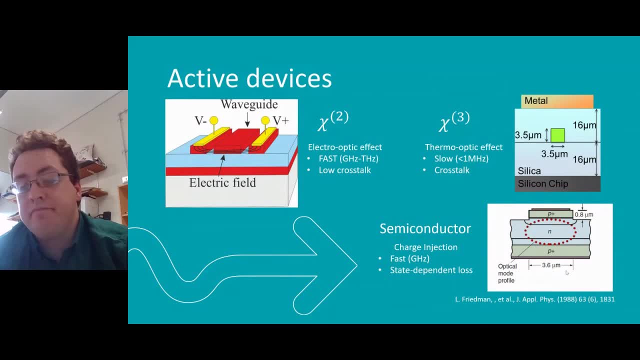 than a Ki2 material. So, using a thermo-optic device to create an active device, we instead deposit a resistor near the waveguide and we just pump heat into the waveguide and with the change in temperature we can change the refractive index As we increase the integration density. this becomes tricky because 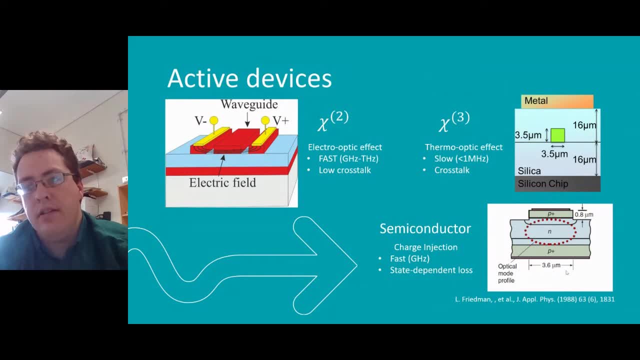 it's a highly sensitive thermal source and there's a lot of cross talk going on and we have to carefully design how to get rid of the cross talk between multiple devices. The other option in semi-conductor materials is to use a charge injection modulator. 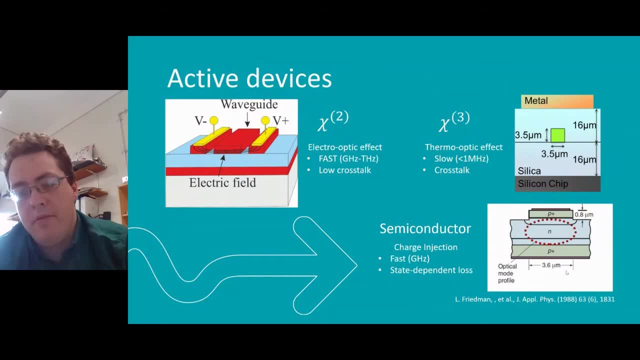 So this is by far the most commonly used in classical photonics because it's extremely fast and it works essentially by creating a pn junction around your waveguard and just pumping charge into your the material where your waveguard is, and this changes the refractive index. but unfortunately for some applications 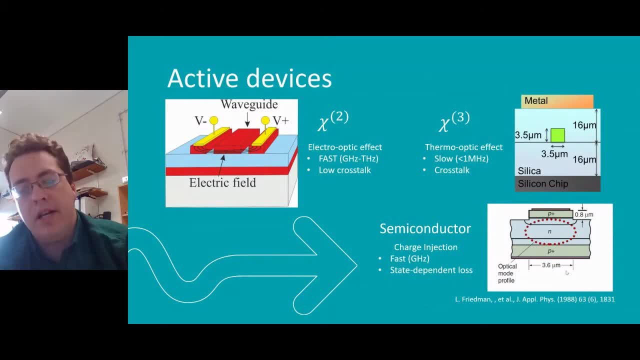 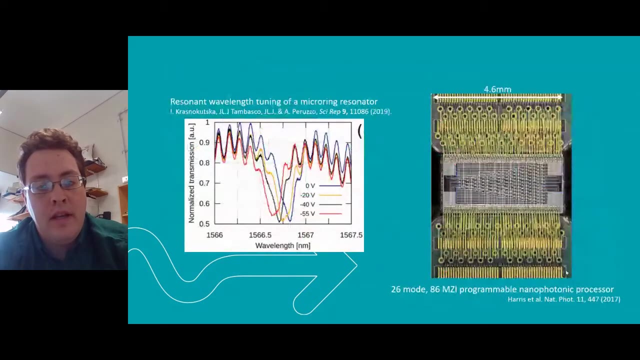 it's not all that suitable because that big dump of electric charge into the region comes with a significantly increased loss. so as an example of a couple of things we can do with these active devices, in a kai 2 material like lithium niobate, the group of alberto peruzzo showed that they can tune the resonance wavelength of a. 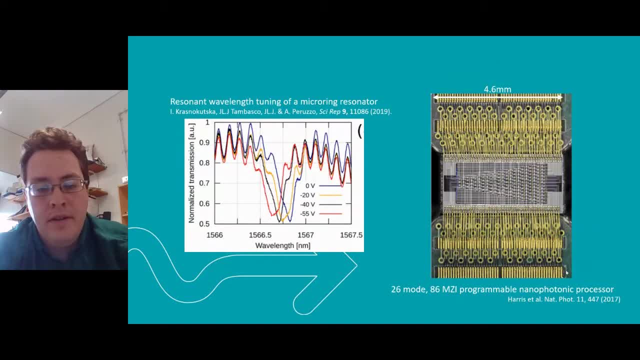 motor and they're able to tune the resonance wavelength of a motor. and they're able to tune the resonance wavelength of a motor and they're able to tune the resonance wavelength of a motor and micro ring resonator using an applied voltage. and, uh, here on the right um is a silicon chip. 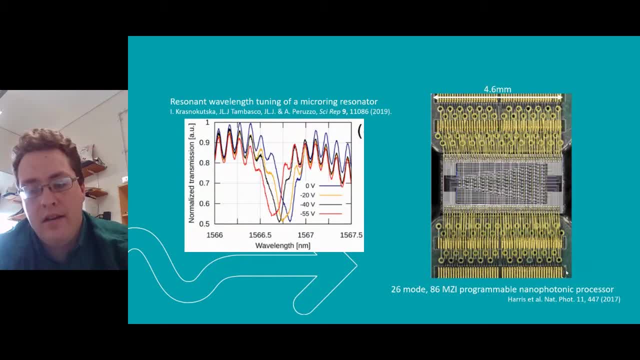 that's a has 26 modes. um, that is completely reconfigurable and it that it sort of shows you the gulf between um sort of the silicon and everything else in that. uh, most other platforms are focused on a few extremely good devices, and silicon is already at this scale of many devices. 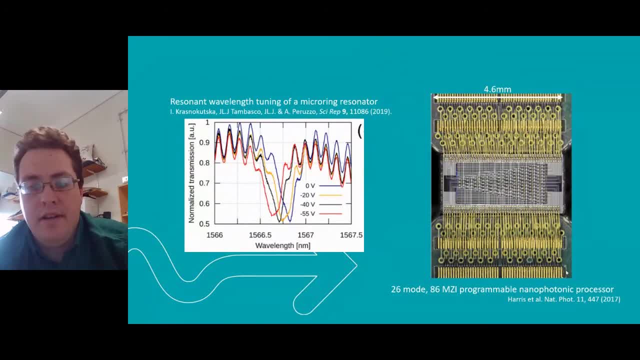 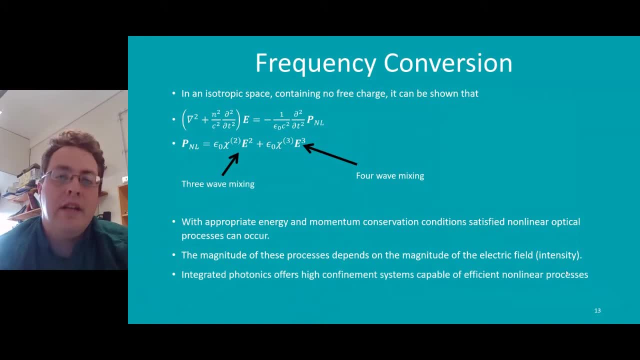 but it's about how well we can functionalize these devices. so, moving on to uh, non-linear effects in these waveguides. so when we uh, when we solve the wave equation, we're going to be able to use the waveguide to solve the wave equation. we're going to 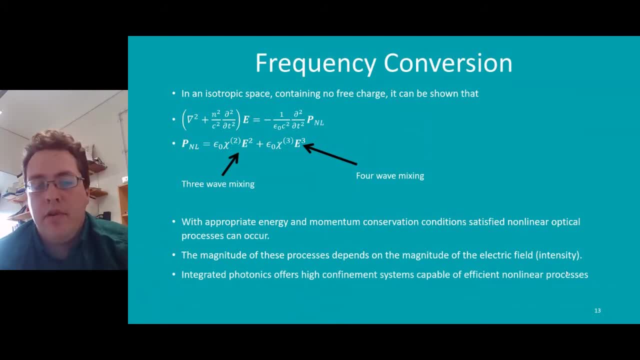 be able to use the wave equation. we've got this uh polarization density term on the on the right hand side and normally we just think of the linear component where we put in one optical field and we get that same optical field back out, the same frequency. instead, in some materials we can get 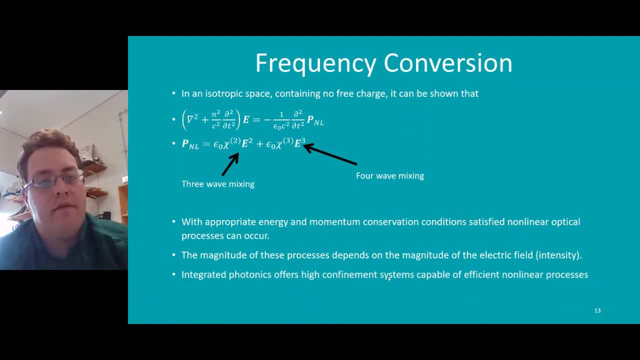 a three wave mixing process where we can change the frequency, uh depending on uh, certain energy and momentum conservation conditions being satisfied. so this is where the chi 2 term comes from, and this is only present in non-centrosymmetric materials. so for centrosymmetric materials, this chi 2 is zero and we're forced to use the next. 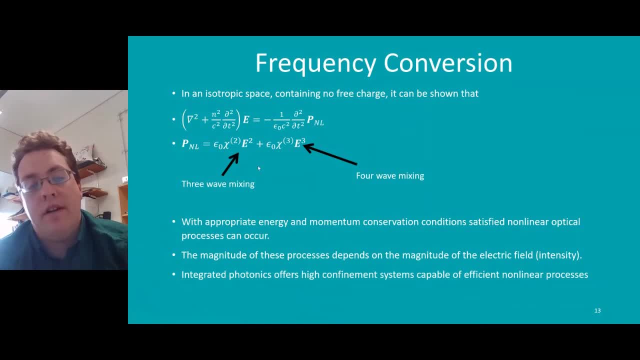 non-linear term, the chi 3 term, which gives us a four wave mixing. why, uh, waveguides are interesting for this field is that the magnitude of these processes depends on the intensity of the optical field, and because we have these high confinement structures, we can create high optical field intensities. 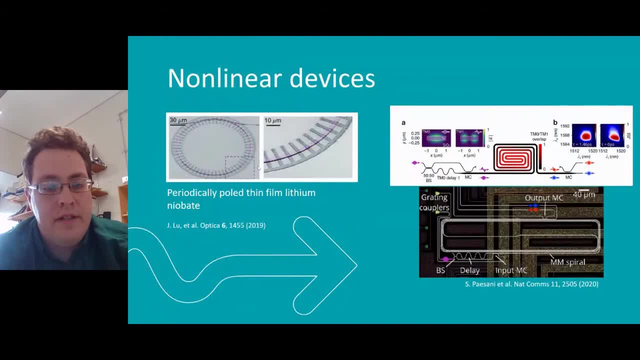 as an example of a couple of these non-linear devices, on the left um we have the periodic polling structure used to create the required uh energy and momentum conservation conditions for frequency conversion in a lithium niobate device, and on the right, we have the phase matching conditions for uh a silicon photonic chip. using this, 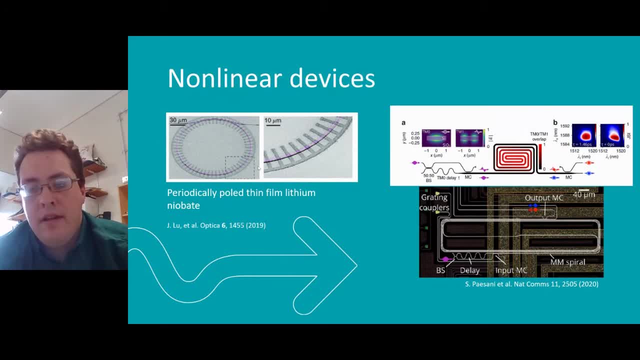 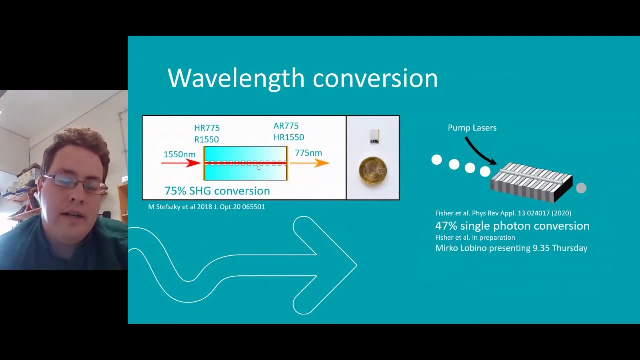 using the chi 3 process, where instead uh, we, they match um these radiating concentration conditions using spatial modes. so what we can do with these high non-linearity devices is that we can perform extremely efficient wavelength conversions. so, for instance, we can get a conversion efficiency much higher than in bulk materials by using a waveguide in a. 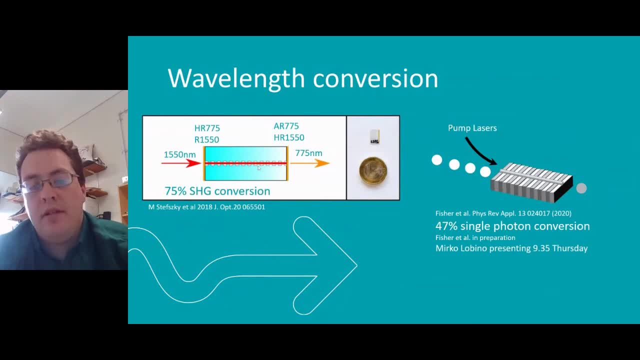 um in a resonator system structure as on the left here to get an extremely high conversion efficiency, And on the right that extremely high conversion efficiency allows us to perform frequency conversion of single photons, So we can take single photons from another region in the telecom spectrum. 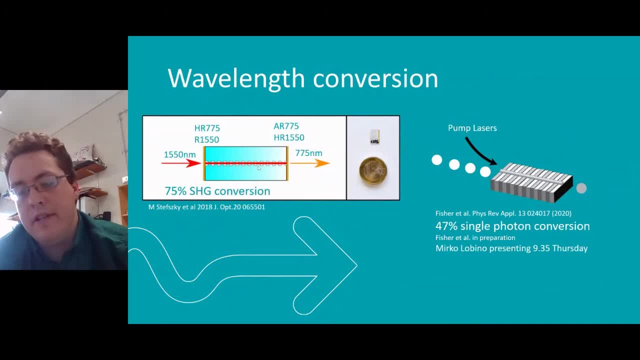 and frequency, convert them using a cascaded process where we first convert up in frequency while simultaneously converting down in frequency to get a small frequency shift till we're at a region of the telecom spectrum that matches up well with a quantum memory, And so Mirko will talk a little bit about this on Thursday. 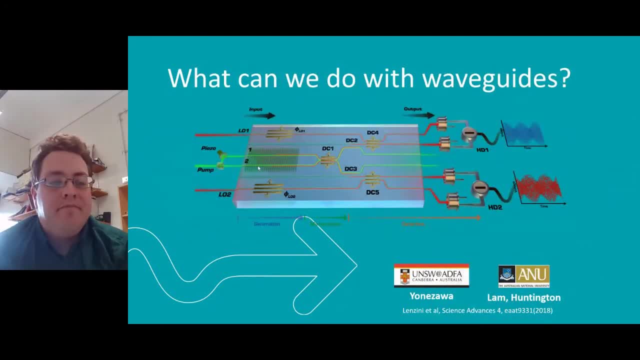 Once we have all these components together, our passive devices and our active devices and our nonlinear devices, And what can we do with them? So one thing we can do, and that we did, was to integrate all of those onto a single photonic chip and create the first demonstration of photonic EPR entanglement. 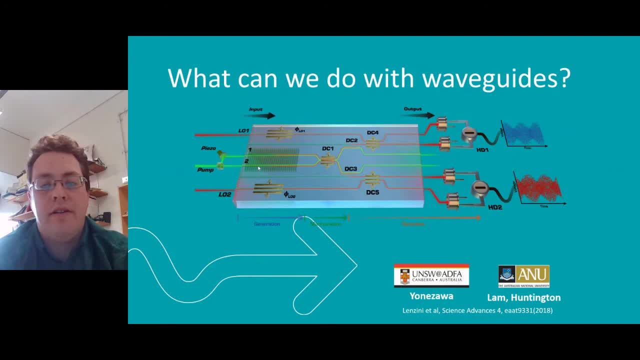 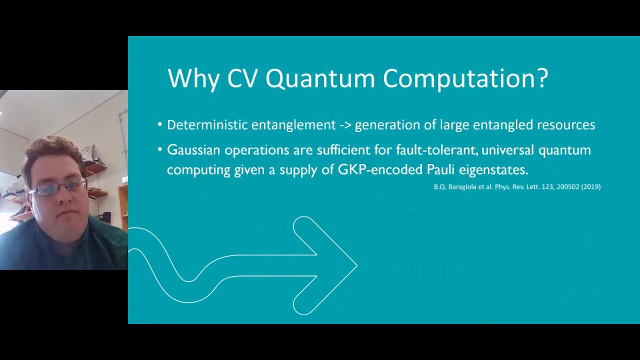 That's generated, manipulated and detected on a single chip. And this leads us to the field of continuous variable quantum optics. and what can integration offer to it? So a couple of sentences on why we're interested in continuous variable computation, especially from a photonic point of view. is that we can access a deterministic 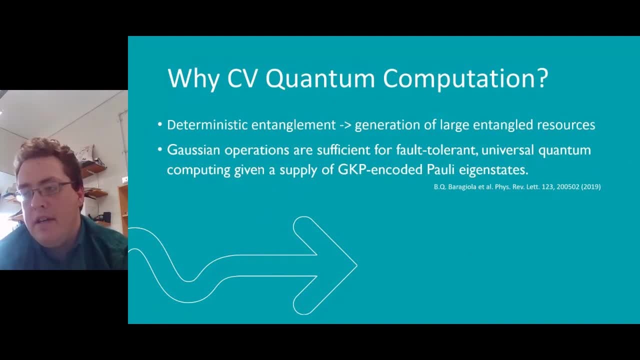 entanglement resource and that gives us the capability of generating large entangled states. And secondly, this nice result from two years ago I guess, shows that with Gaussian operations we can perform, we can have a fault tolerant universal quantum computer. 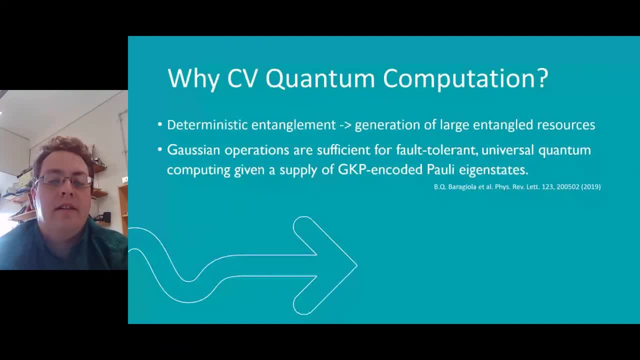 given a supply of GKP encoded Pauli eigenstates, So I won't talk about these GKP states, but I will go over a little bit about these Gaussian operations and how we might implement something useful for continuous variable quantum computation in an integrated class. 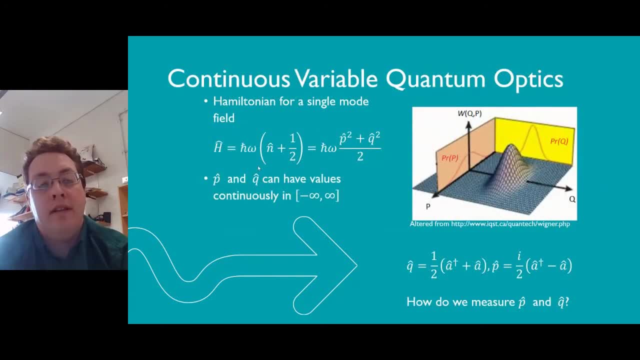 So let's take a look at some of the data that we've got here. So to step back a little bit into what do I mean by continuous variables, So single mode of a quantum harmonic oscillator. Normally the way we talk about it is with the excitation number. 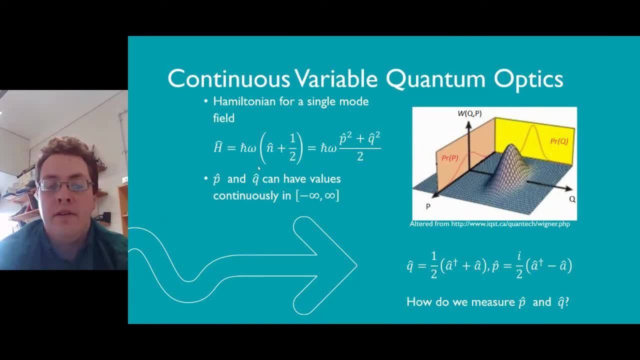 So the number of photons- this N term here, but we can equivalently describe it using the quadrature operators P and Q, And the reason it's called continuous variable is that these have values anywhere in the range from minus infinity to infinity. 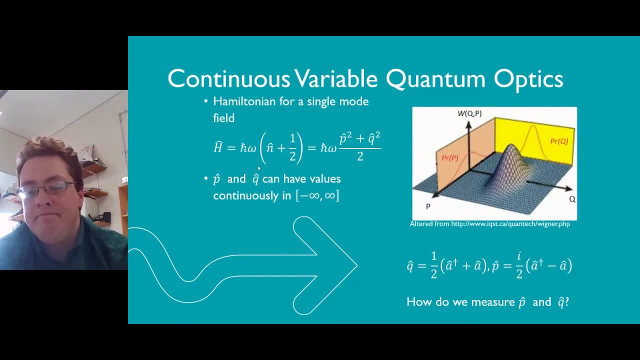 And we can plot these values on a Wigner function plot And that'll show us the quasi probability distribution of our state. So we can see the probability of a certain Q or P value occurring. And then the question is, how do we measure these values? 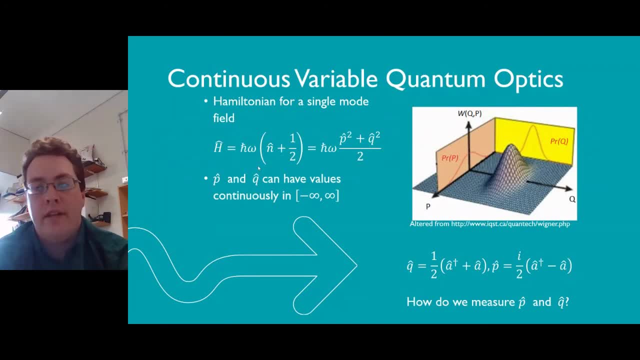 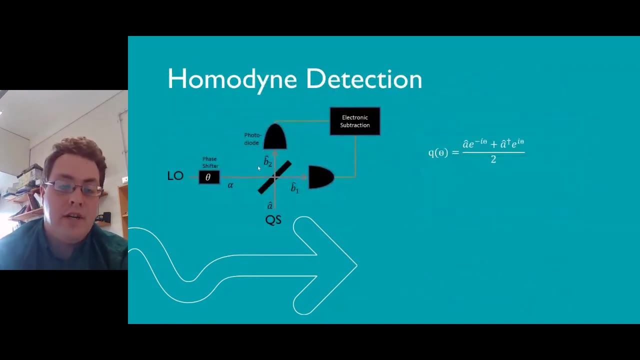 For excitation number. it's fairly simple. We can use a single photon detector or a photodiode measures this value. To measure quadrature values we use a homodyne detector. So in a homodyne detector we start with our quantum state on one arm. 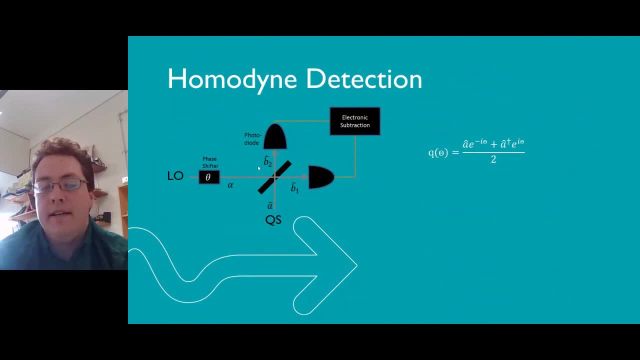 and a strong classical field called the local oscillator on the other arm. We combine them on 5050 beam splitter and send the output to two photodiodes And the current of these two photodiodes is subtracted. The output of these- no subtraction- is proportional to the quadrature operators. 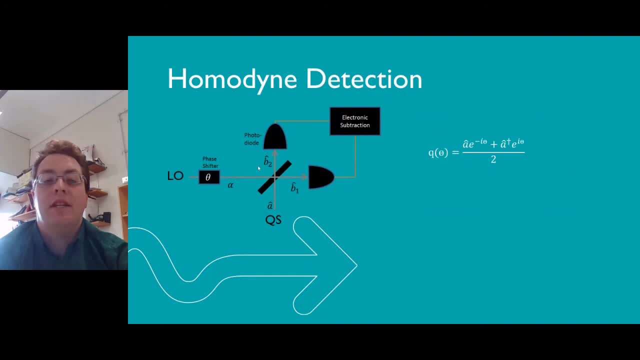 And if we set the relative phrase between the quantum state and the local oscillator to zero, we can measure the Q quadrature. And if we set it to pi on two, statistically that can go directly to prime greater. And if we put it to pi on two then we can measure a W inspired Sell Jahren. yeah. 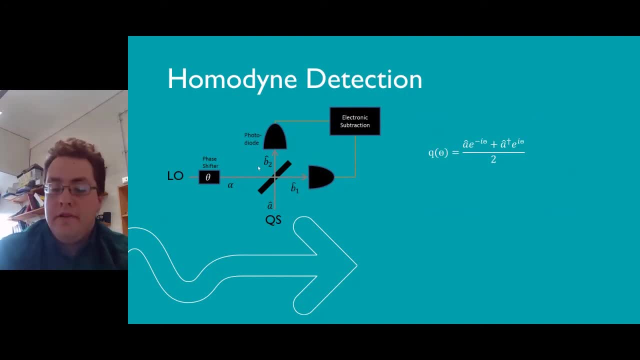 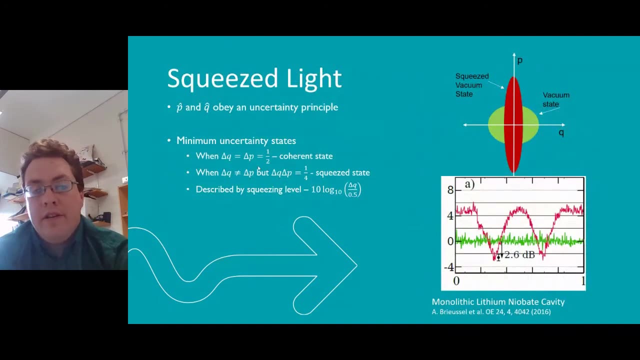 So the quantum state toмерize, so you can measure mixing ratio it to pi on two we can measure the p quadrature. One of the fundamental resources of continuous variables is the squeeze state. So these quadrature operators, p and q, are an uncertainty principle. 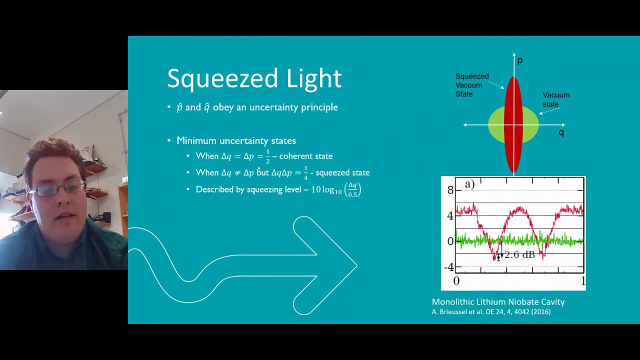 and that means we can talk about a minimum uncertainty state. So we have a vacuum state or a coherent state is a minimum uncertainty state where the uncertainty in position and momentum q and p are equal. But if we instead reduce the uncertainty in one of these, 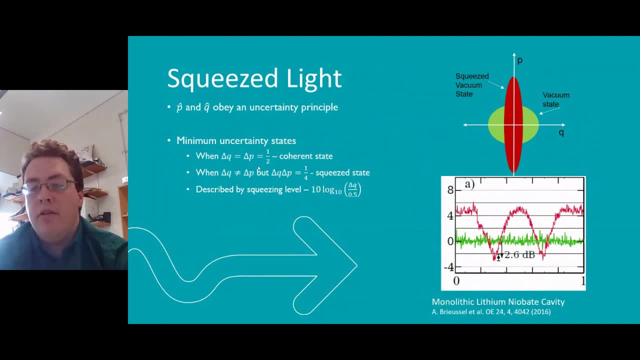 quadratures at the expense of increasing the uncertainty. in the other quadrature we create a squeeze state, which is a minimum uncertainty state, And that means that in the one quadrature where we've reduced the uncertainty we can actually reduce the uncertainty below the shot noise level. So from the plot on the right you can imagine: 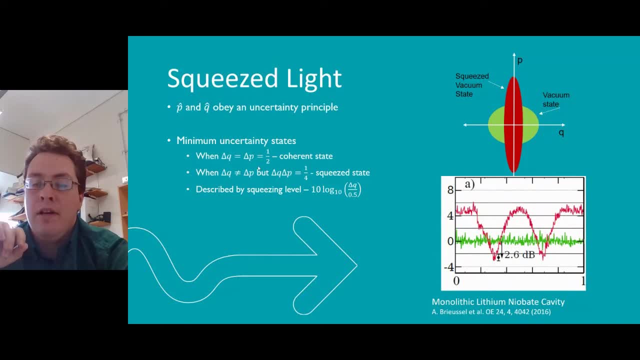 it as rotating around the diagram at the top. So the vertical axis is the sort of the variance and you can see that if you look at it straight down from the top, we get a very narrow variance in our state, in our red state there, compared to our green state. 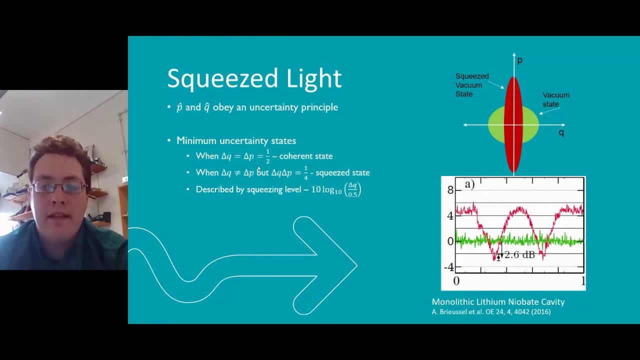 And so that's less than the shot noise level. If we then rotate around to looking at it from the left or right, the variance is a lot larger than vacuum state, And so the red line shoots above the green line again, And if we keep rotating around we keep getting. 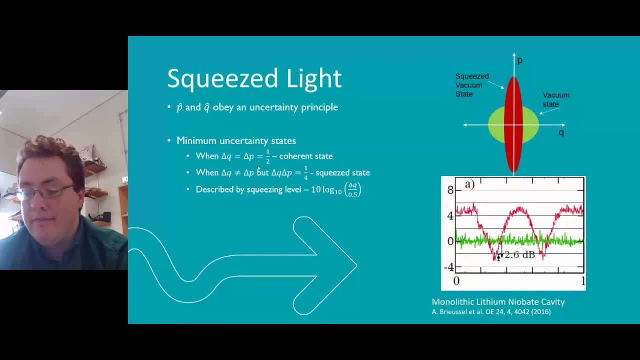 more and more of the same thing, And so that's what we're trying to do here. So we're going to go back to the plot and we're going to go back to the rest of that plot. Ben, you have about four minutes to go. 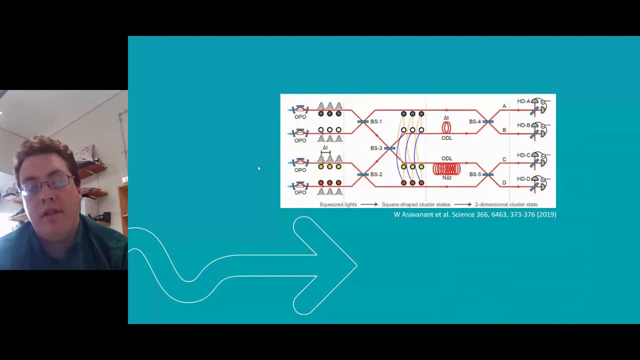 So in bulk optics the great experimental demonstrations so far have been from the group of Akira Furuzawa and there's another similar one from the group of Anderson. So you can see that the difference between the two is really, that it's not just a. 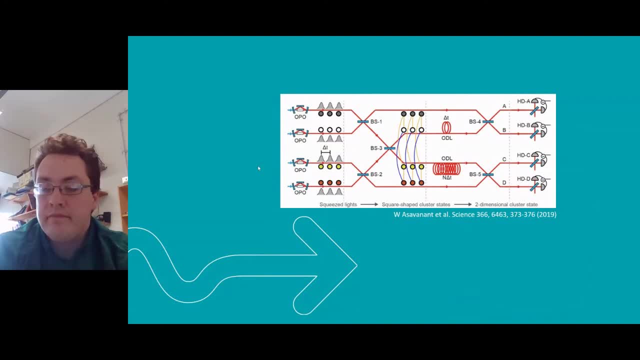 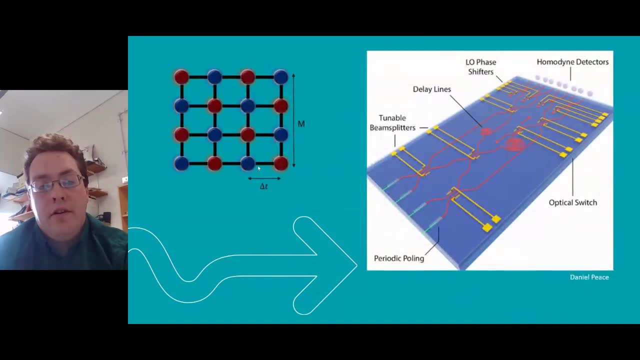 small number of objects, but it's a very large number of objects And you can see that there's a lot of space between them. So we're going to go back to the plot and then we're going to go back into the plot and we're going to go back to the real thing. 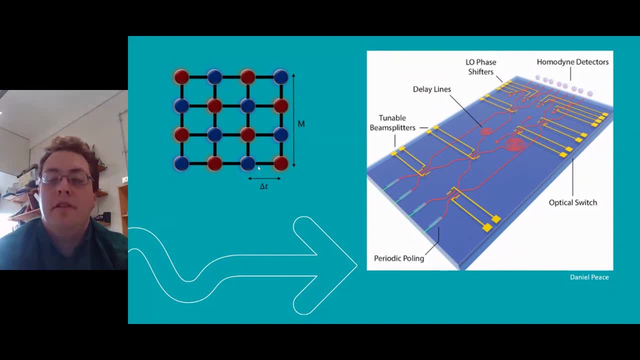 So you can see that there's a lot of space, dimension is spatial and the horizontal is time, and so what we can move towards in integrated photonics, given our ability to have these non-linear devices and these active devices, is that we can move towards integrating this whole thing, which takes up a benchtop or more. 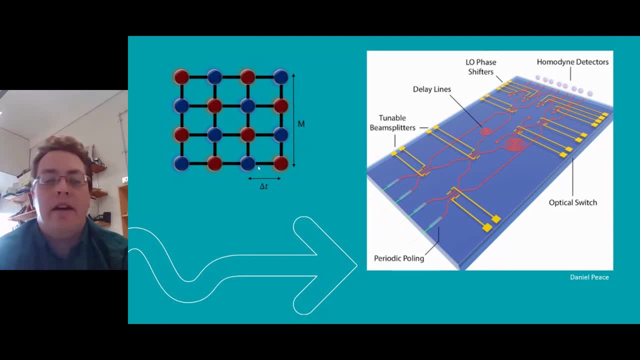 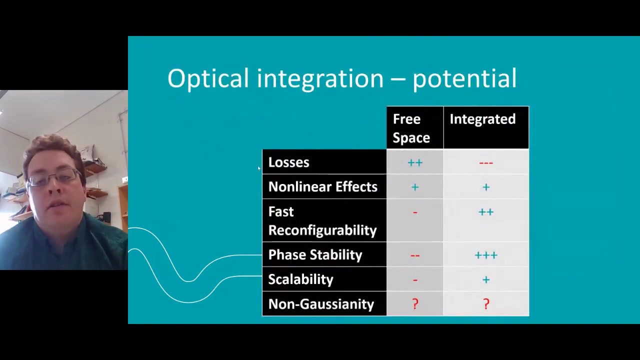 into a single package, as as illustrated on the right here. so, starting at the bottom, we have our non-linear regions and we go through a variety of active devices to mimic the bulk setup before going to our detectors at the end. so why we want to move towards this sort of goal is that